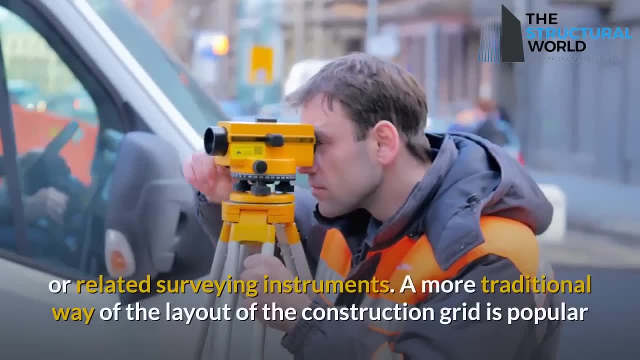 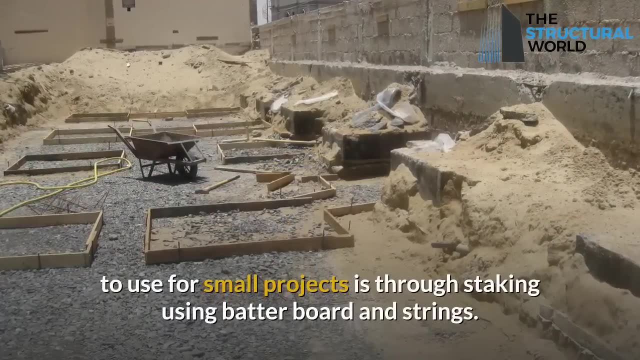 the construction grids can be layout through the use of theodolite or related surveying instruments. A more traditional way of the layout of the construction grid is popular to use for small projects is through staking using batter board and strings. Batter board are temporary wooden. 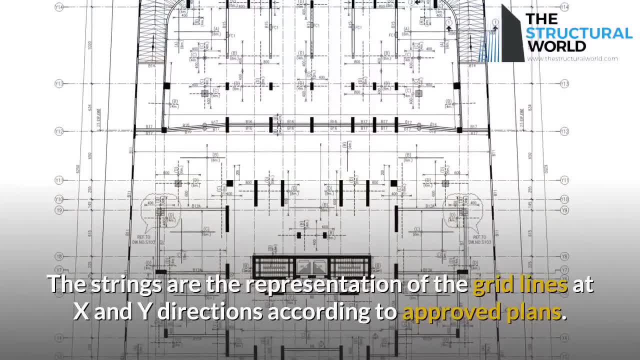 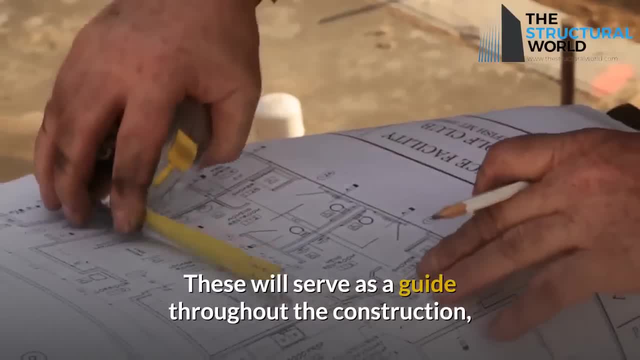 frames used to suspend the strings. The strings are the representation of the grid lines at x and y directions, according to approved plans. These will serve as a guide throughout the construction, so it is important to fix a reference line in both directions, to be used once the grids have. 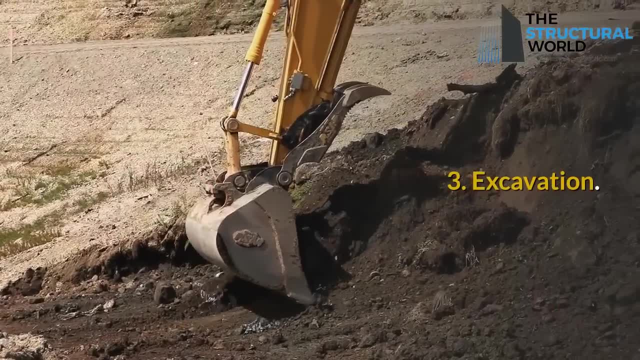 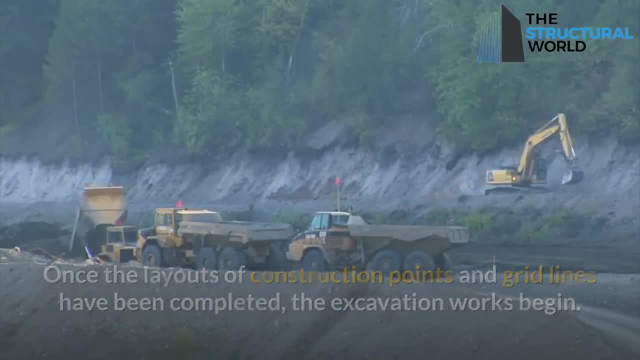 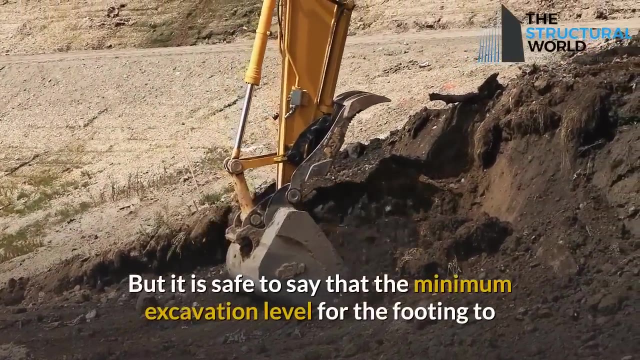 been placed, when needed, in the construction. 3. Excavation: Once the layouts of construction points and grid lines have been completed, the excavation works begin. The excavation depth depends on the recommendation by the soil investigation report, But it is safe to say that the minimum excavation level for the footing to rest should stick to 1. 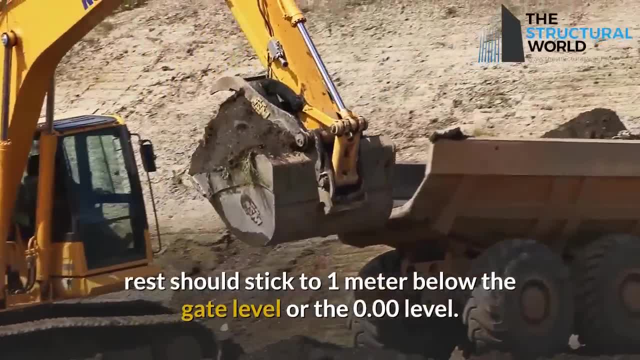 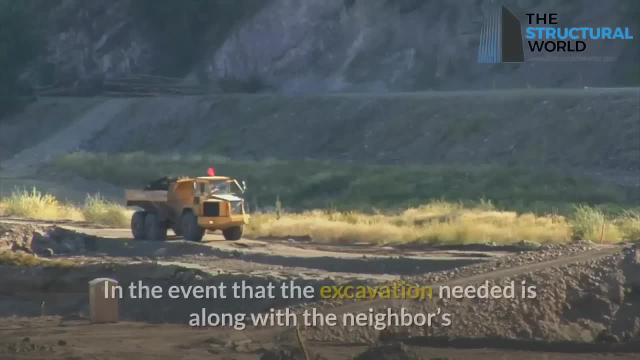 meter below the gate level or the 0.00 level. Excavation works is a massive activity. therefore, a proper caution should be observed during this stage. In the event that the excavation needed is along with the neighbor's existing structure, the excavation works should. 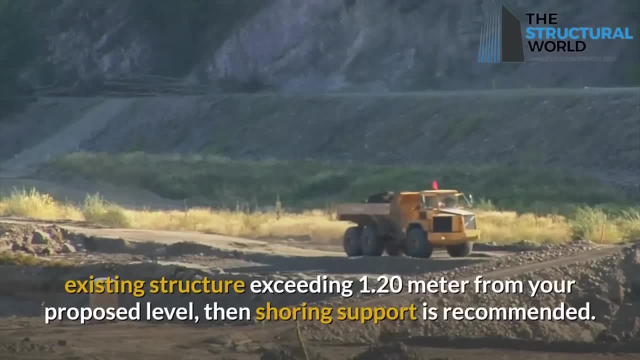 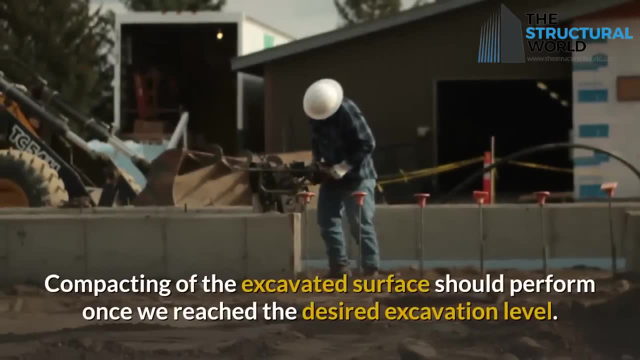 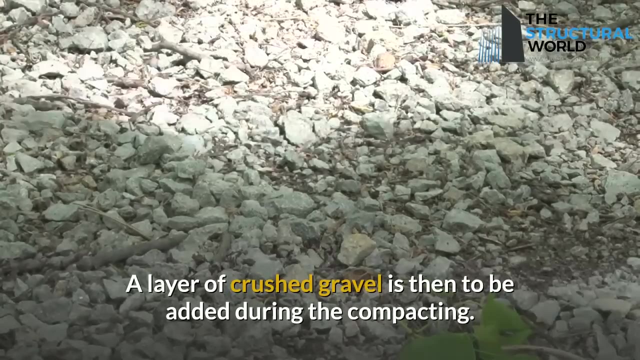 be done at a depth of 1.20 meter above the proposed level. 4. Compacting and laying of PCC. Compacting of the excavated surface should perform once we reach the desired excavation level. A layer of crushed gravel is then to be added during the 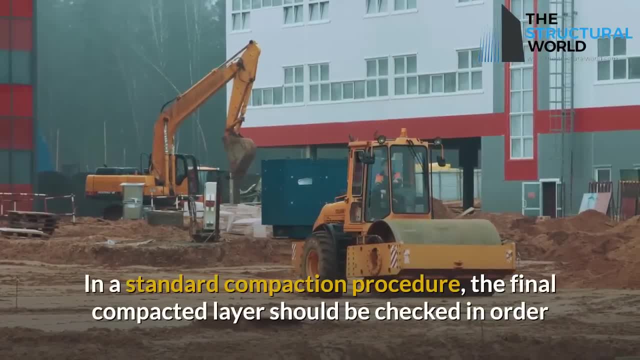 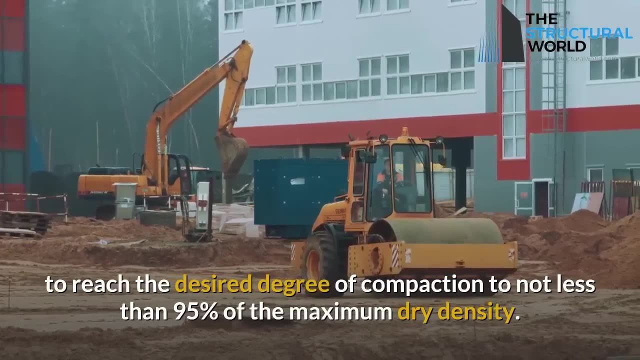 compacting In a standard compaction procedure, the final compacted layer should be checked in order to reach the desired degree of compaction to not less than 95 percent of the maximum dry density. It is then in this stage that an anti-termite treatment on the ground should also be considered. 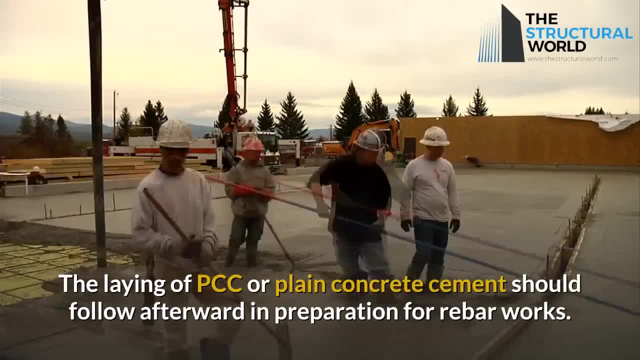 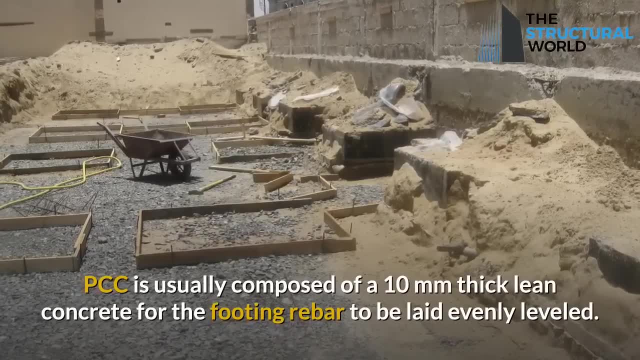 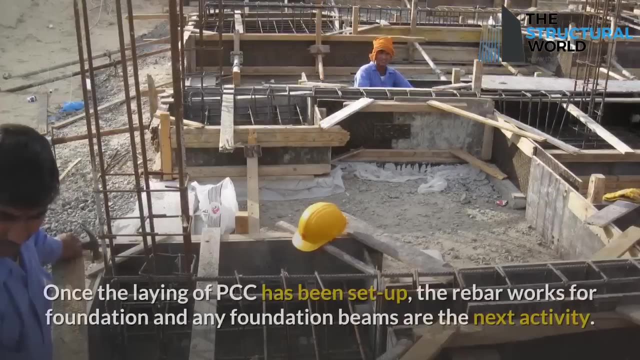 The laying of PCC or plain concrete cement should follow afterward in preparation for rebar works. PCC is usually composed of a 10 millimeters thick lean concrete for the footing rebar to be laid evenly leveled. 5. Foundation rebar and column starter bars Once the laying of PCC has been. 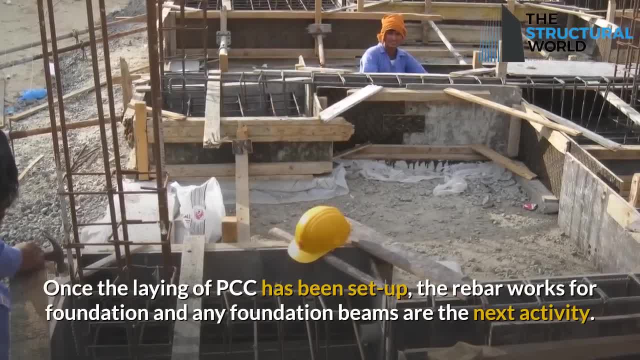 set up. the rebar works for foundation and any foundation beams are the next activity In this stage. the rebar works for foundation and any foundation beams are the next activity In this stage. the rebar works for foundation and any foundation beams are the next activity. 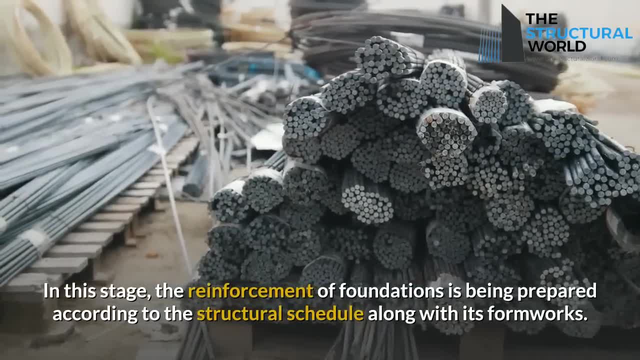 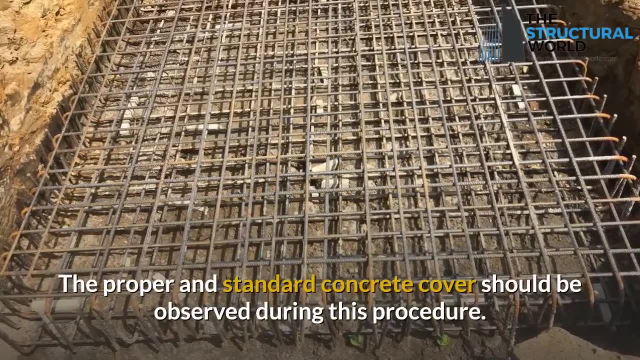 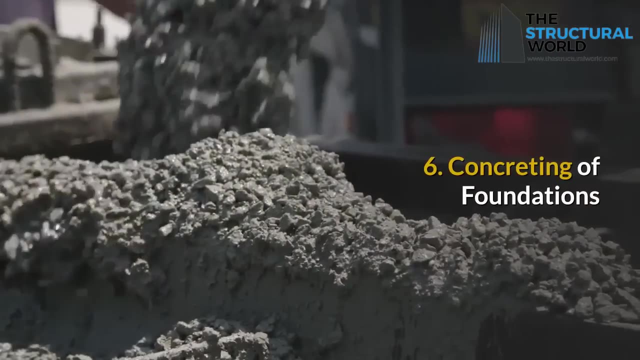 In this stage, the reinforcement of foundations is being prepared according to the structural schedule, along with its formworks. The proper and standard concrete cover should be observed during this procedure. Starter bars for columns should also be installed accordingly before concrete pouring. 6. Concreting of foundations and column rebar installation. Concreting of foundations has 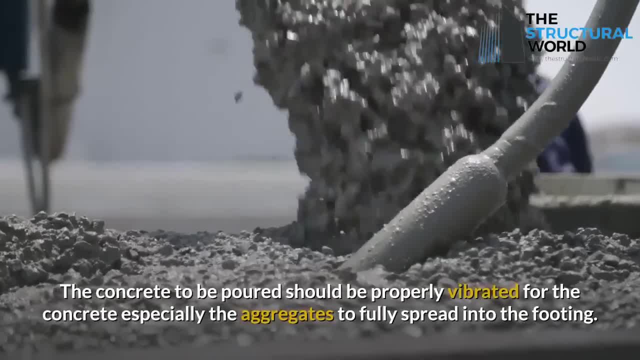 to come next, after the rebar works. The concrete to be poured should be properly vibrated for the concrete, especially the aggregates to form the foundation. The concrete to be poured should be properly vibrated for the foundation. The concrete to be poured should be properly vibrated for the. 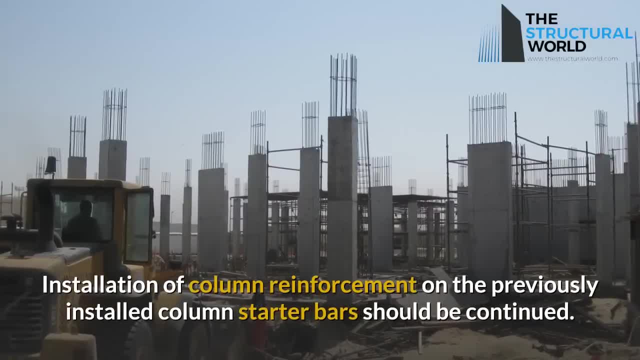 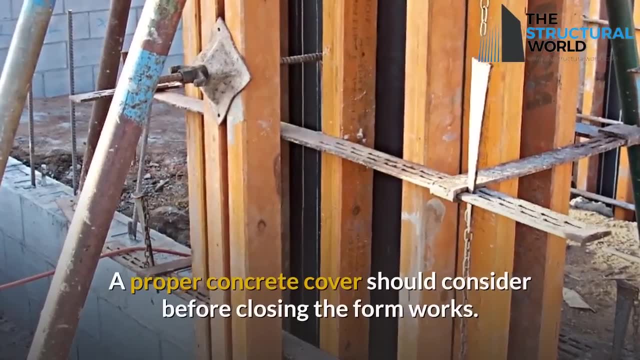 foundation. The concrete to be poured should be properly vibrated for the foundation. Installation of column reinforcement on the previously installed column starter bars should be continued. A proper concrete cover should consider before closing the formworks. For substructure columns an additional concrete cover of at least 50 millimeters has to be considered up to plinth. 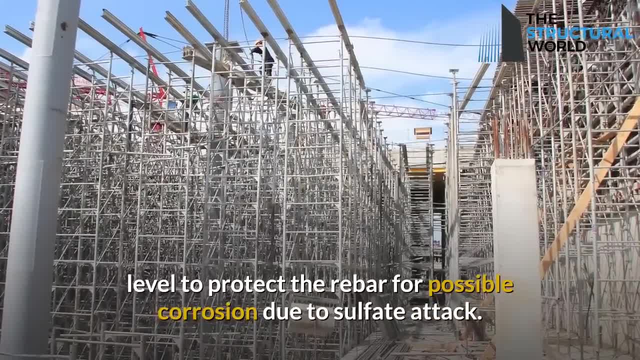 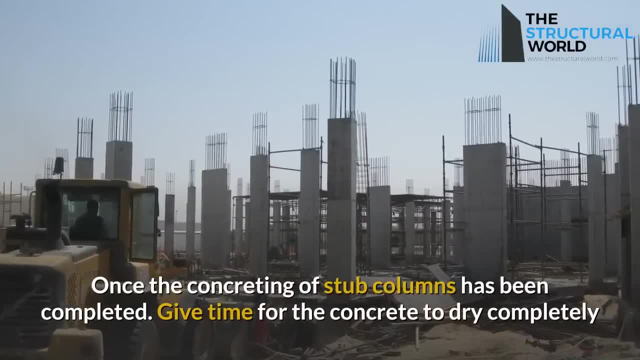 level to protect the rebar for possible corrosion due to sulfate attack. 7. Concreting of column and bitumen paint applications. Once the concreting of stubbed columns has been completed, the concrete must sourced completely of the inside and outside edges and beaten to perform crops, Give time for the concrete to dry completely and apply at least two coats of bitumen. 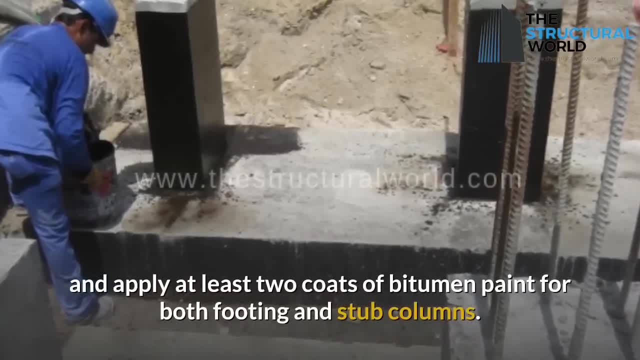 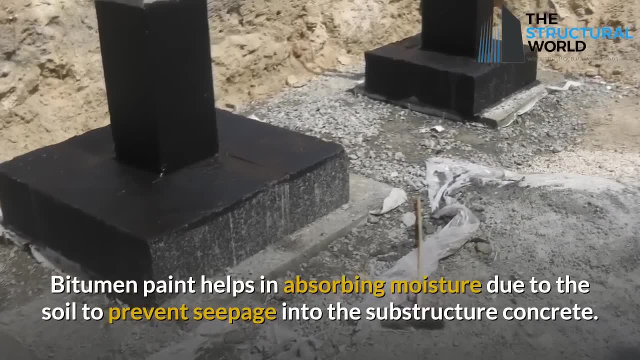 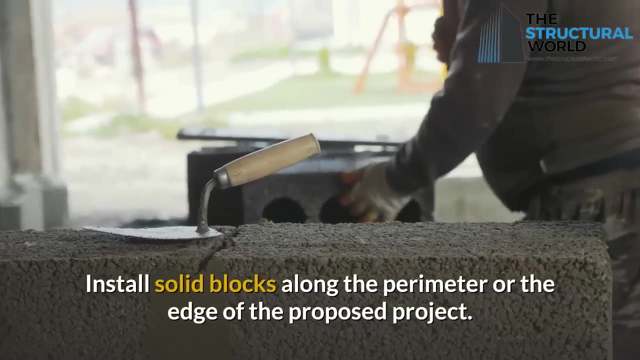 paint for both footing and bitumen paint helps in absorbing moisture due to the soil. to prevent See Χ into the substructure, concrete loan blocks a problem on the perimeter or the edge of the proposed project. This is to establish a boundary between the inside and outside edges of c. 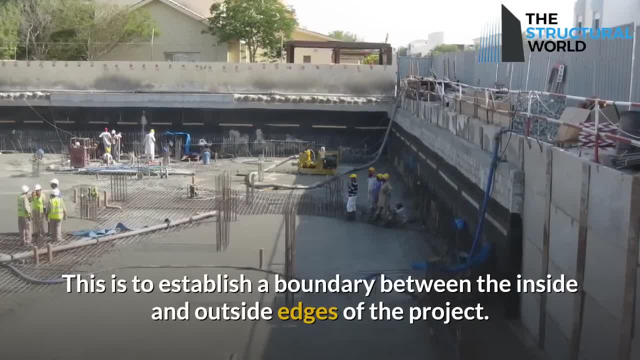 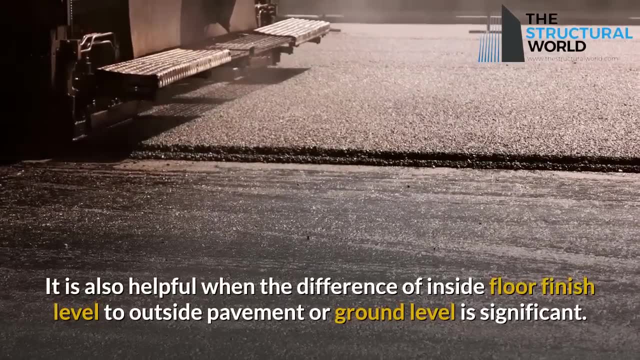 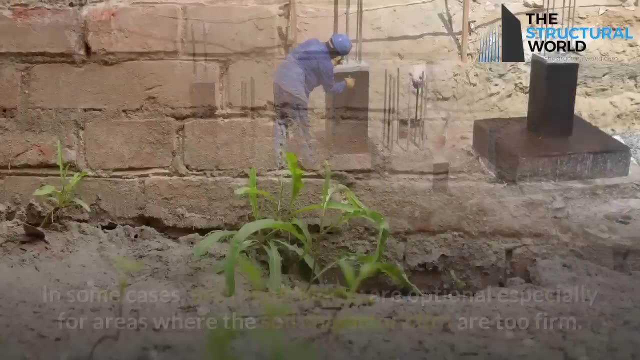 of the proposed project. It is also helpful when the inside floor setting off blocks inside finish fittings flooring level. This, the finished å, the wire must be winked around. the outside pavement or ground level is significant. two coats of bitumen paints should also apply afterward. in some cases perimeter blocks are optional, especially for areas where the soil 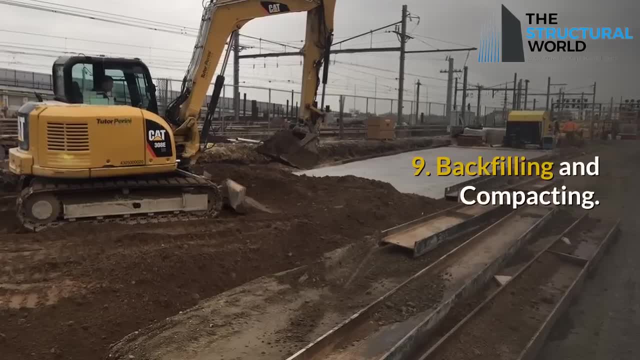 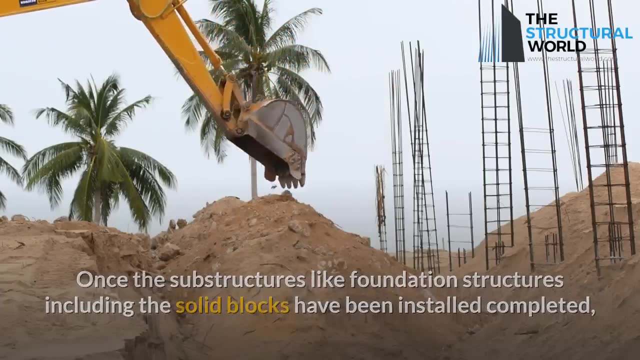 characteristics are too firm. 9. back filling and compacting. once the substructures, like foundation structures, including the solid blocks, have been installed completed, backfilling and compacting should take place. backfilling and compacting should be done partially to make sure that the